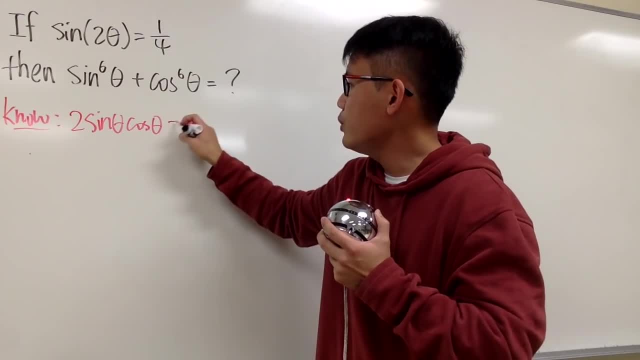 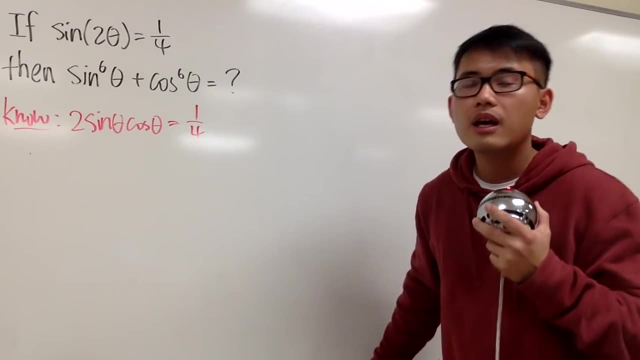 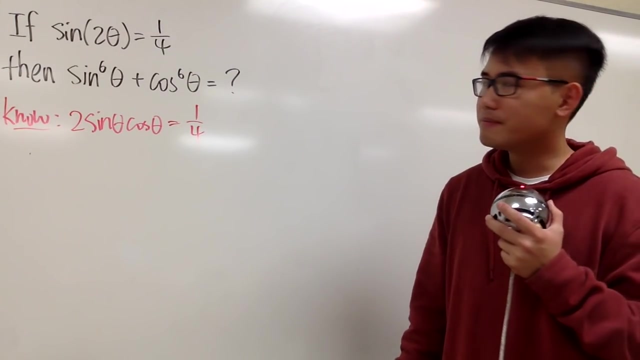 are the same and of course, this will be still equal to 1 over 4.. Okay, and now let's look at this carefully: Sine to the 6th power plus cosine to the 6th power. It looks kind of suspicious: the 6th power, and in fact I think I know how to factor this out. 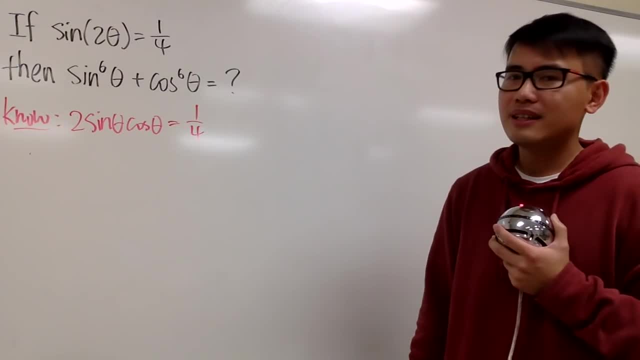 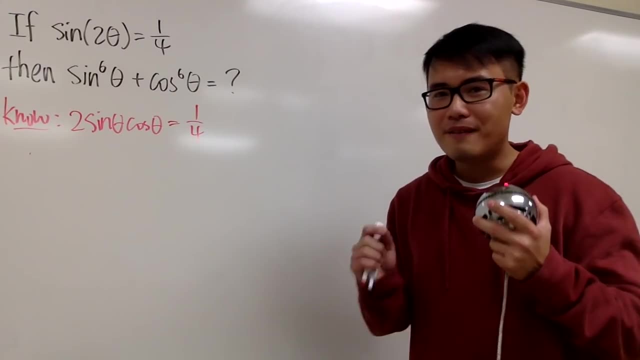 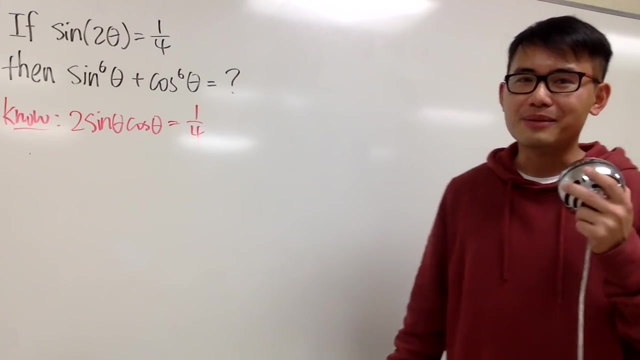 because we have done something like that in algebra, right. But then to factor out 6th power, we cannot do this right away because we only can factor the sum of two cubes. We cannot factor out the sum of two squares, but we can factor out the sum of two cubes, right. So let me put down that. 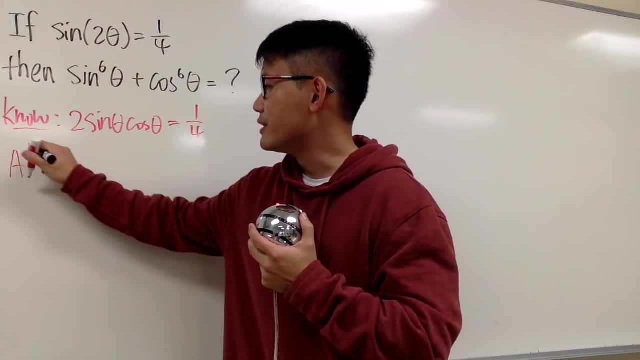 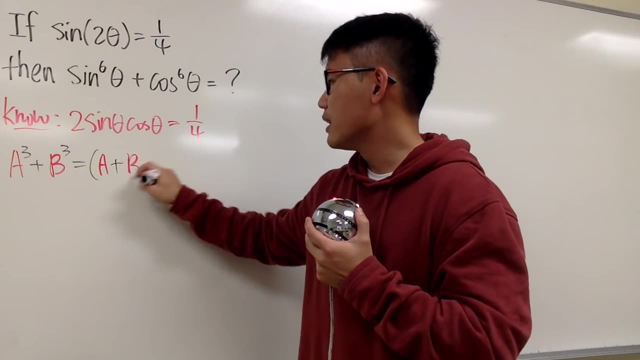 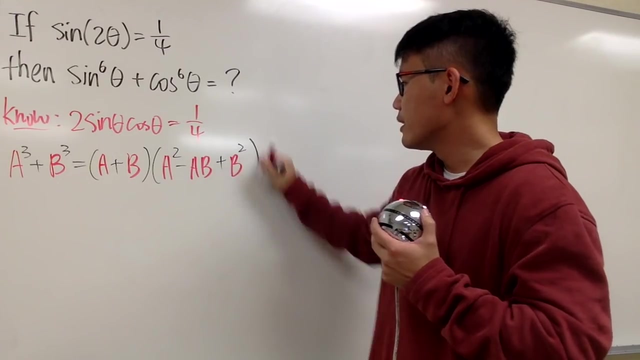 this is what we know as well. If we have a to the 3rd power plus b to the 3rd power, this will be the same as a plus b, and then we multiply by a squared minus a- b, and then plus b squared like. 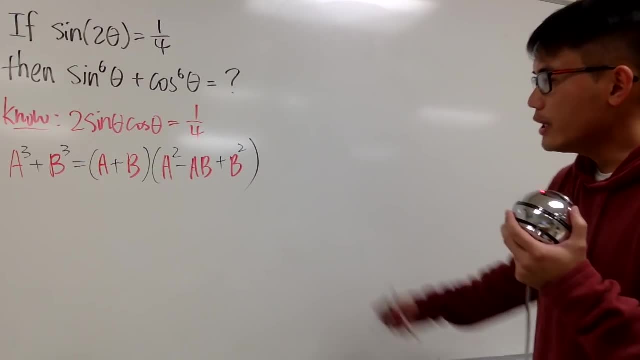 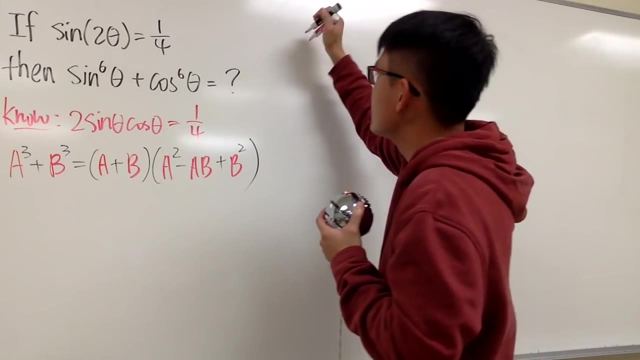 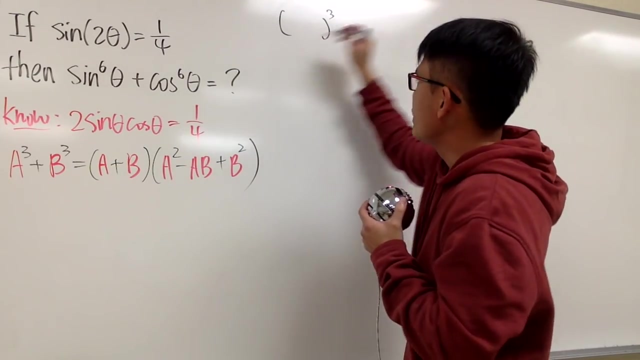 that right. So why don't we try to use this formula and try to factor this out and try to break it down as much as possible- and let's see what will happen- and put it down right here for you guys To factor this out, I will have to write this as something to the 3rd power and then we add with: 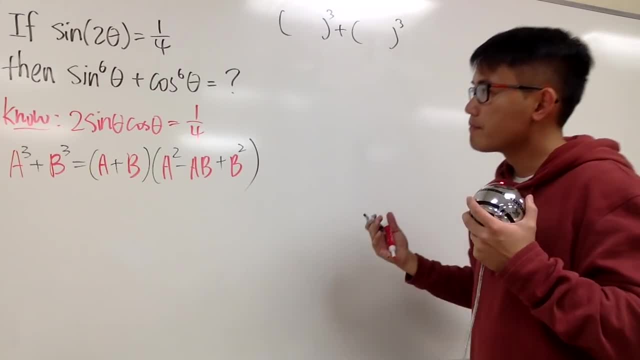 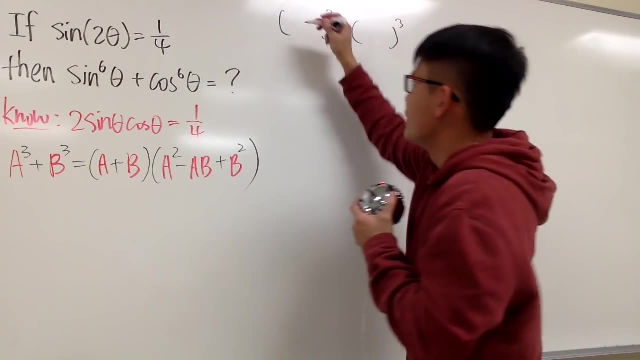 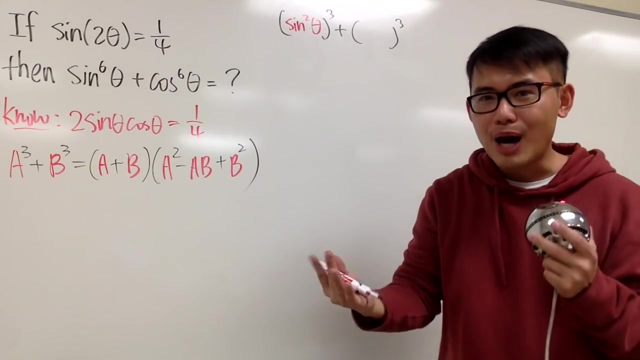 something else to the 3rd power, right? Well, first we have sine to the 6th power theta. What should I fill in in the parentheses? Okay, I can just fill in this as sine squared theta, because the 2nd power and then raise to the 3rd power. we multiply the powers 2 times 3, we get 6, right. So similarly, 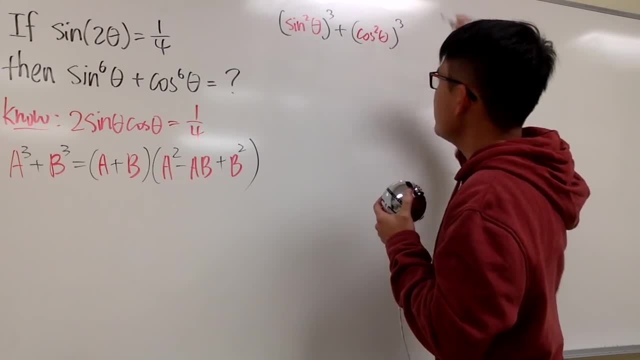 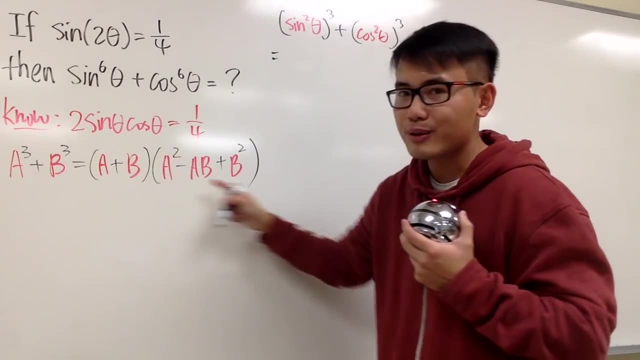 right here, we need to have cosine to the 3rd power. So let's do it sine squared theta. And now we can get to work, because this is the a, this is the b, So let's go ahead and factor it out right here. okay, So we will have a plus b, which is going to be sine. 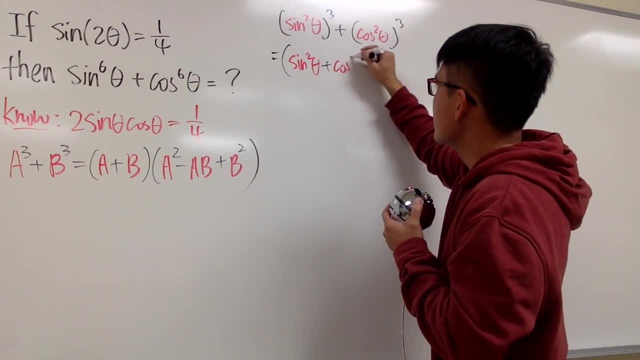 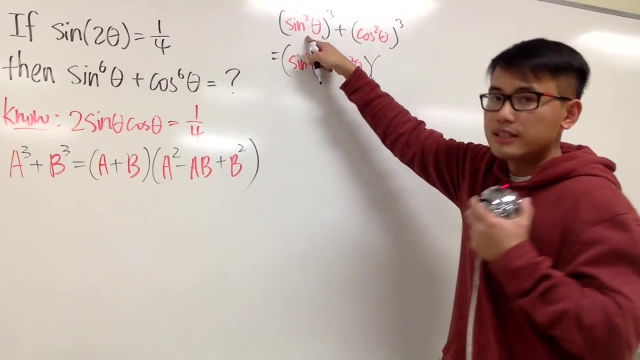 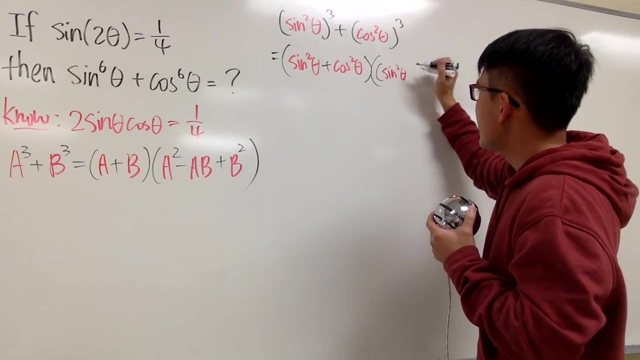 squared theta plus b, which is cosine squared theta, And then for the second parentheses, we will have a squared, which is this, and then squared. And let me write this down for you guys: first I will put it down as parentheses: sine squared theta, and then squared, and then minus. 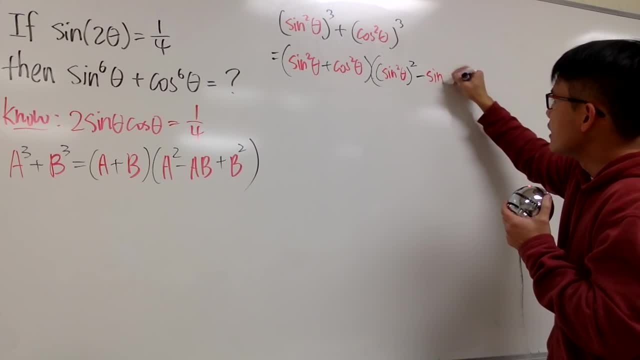 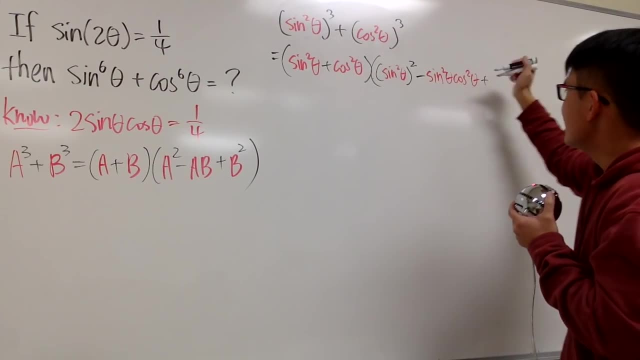 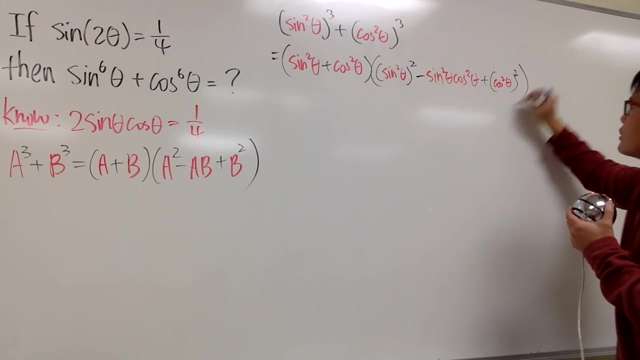 a, b, which is this times that sine squared theta, cosine squared theta, and lastly, we have that plus b squared, And once again, let me keep a parentheses around it- cosine squared inside like this and then squared that, And this is what we have. How cool is this. 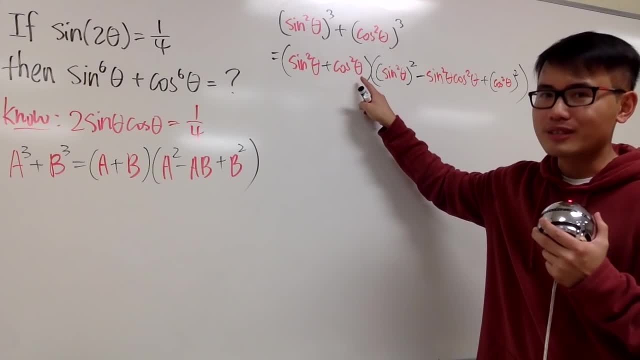 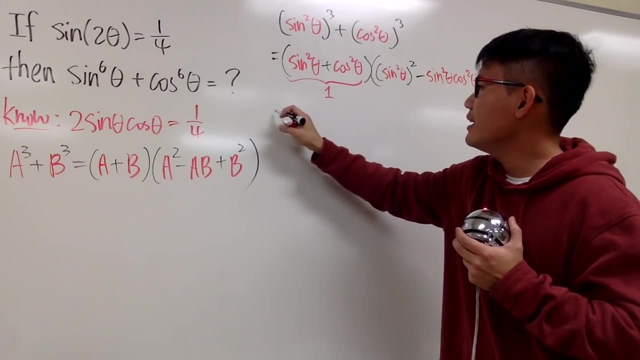 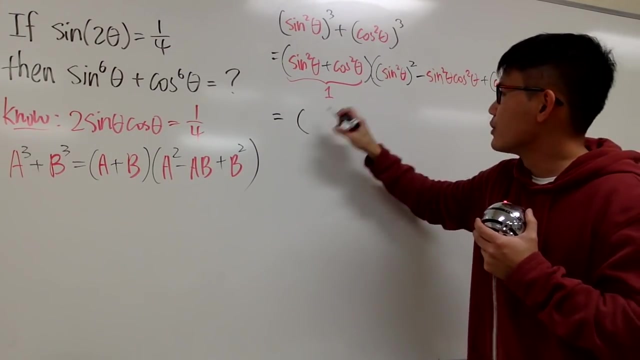 You see that. You see that already. huh, Because sine squared theta plus cosine squared theta is nothing but just one, isn't it? So this right here is just one and one times this. Of course, we just have this to work with right. Let me write this down again: This is just going to be sine squared theta. 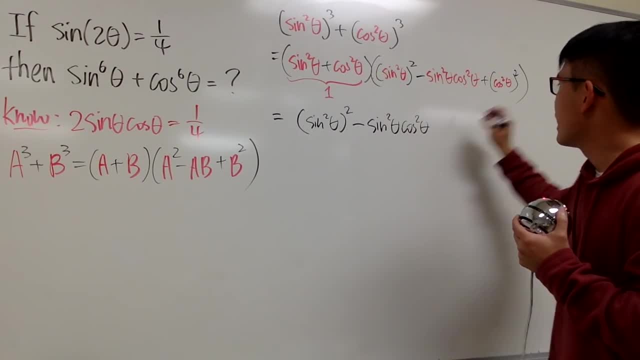 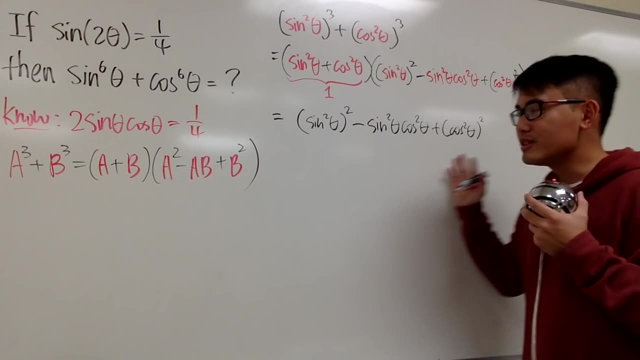 squared, minus sine squared theta, cosine squared theta. and then, plus parentheses, cosine squared, theta squared. I know this is sine to the fourth power theta, but let me just keep it as a whole. So this is sine squared theta plus cosine squared theta squared. minus sine squared. 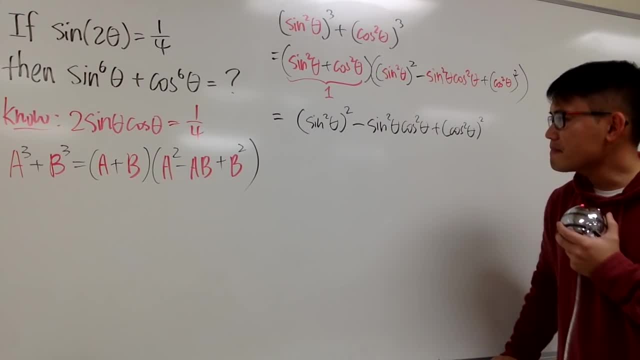 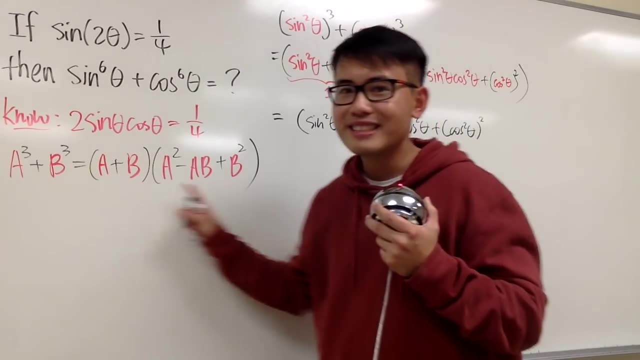 theta squared. and then plus sine- squared- theta squared. minus sine squared- theta squared. and then plus sine- squared- theta squared. and then plus sine- squared- theta squared. and then how it is. Okay, This is really nice. And can we still keep factoring? Well, this formula stops. 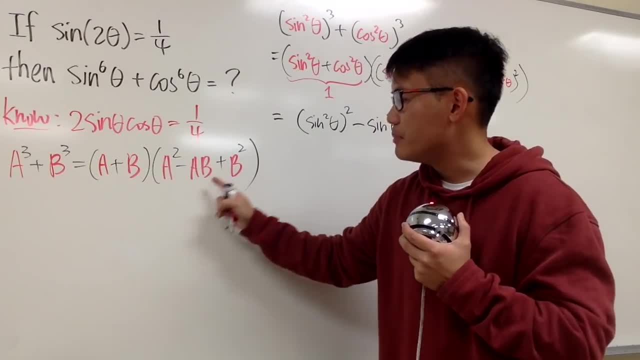 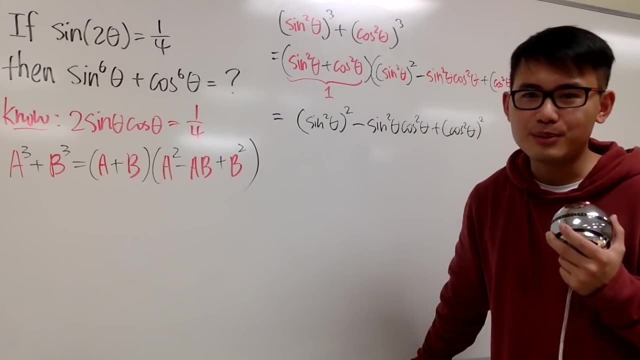 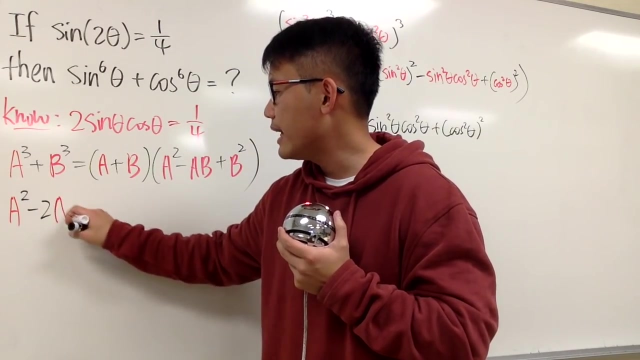 right here, because this is not factorable: a squared minus a, b plus b squared. we know this is not factorable, right? However, we know something similar and that's actually factorable. Let me write it down. We first know that if we have a to the second power minus 2, a, b. 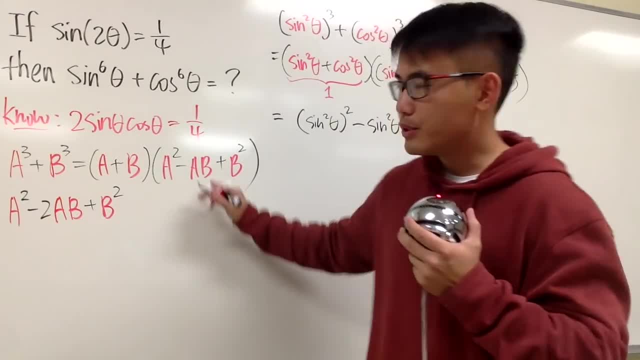 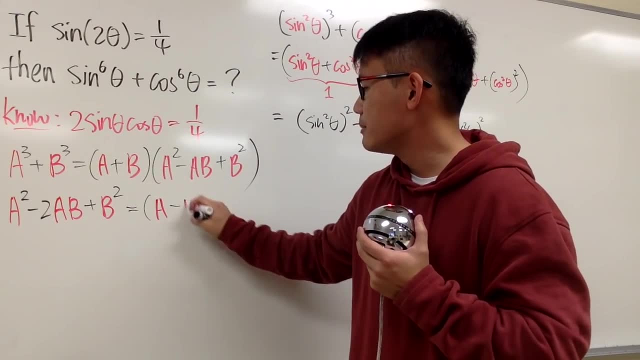 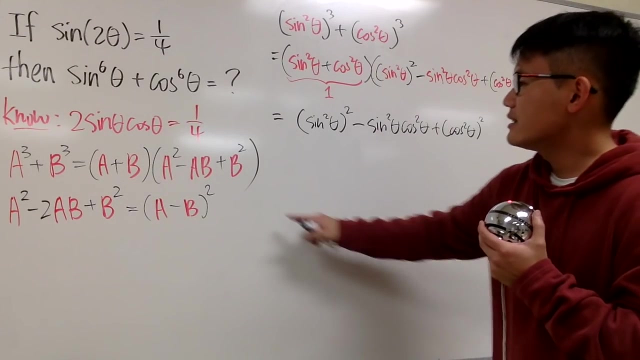 and then plus b squared. huh, this is similar to that right And this is actually factorable. This is the same as saying we will just have a minus b n squared. That's nice right. And you see, a is this, b is that the sine squared theta, cosine squared theta? In fact, I don't. 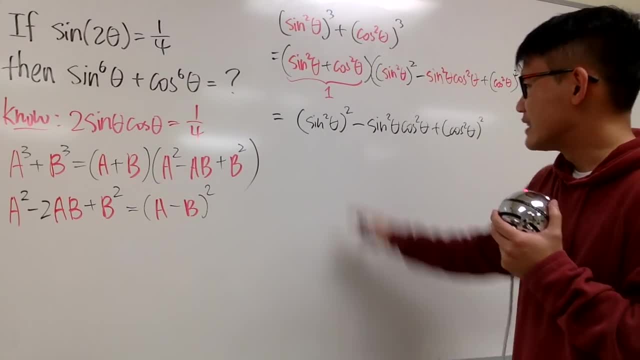 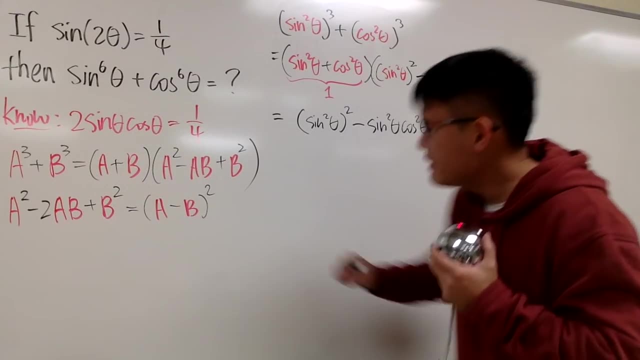 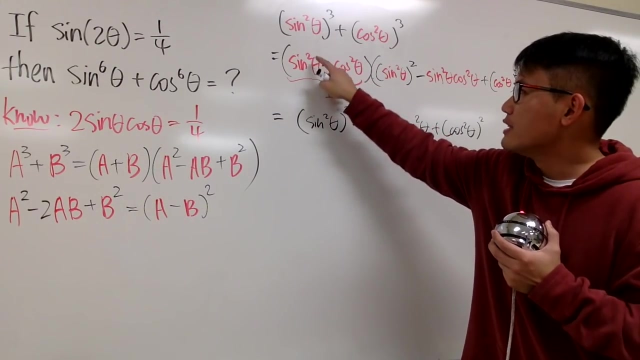 really want to use this formula because, as I said, this is the a, this is the b. If I happen to end up with sine squared theta minus cosine squared theta, I don't know too much about it. right? This is much better. Sine squared theta plus cosine squared theta is. 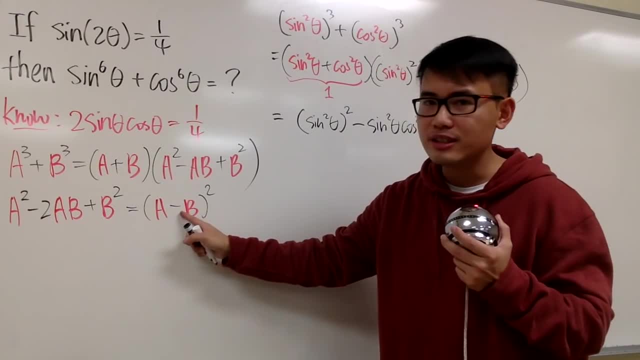 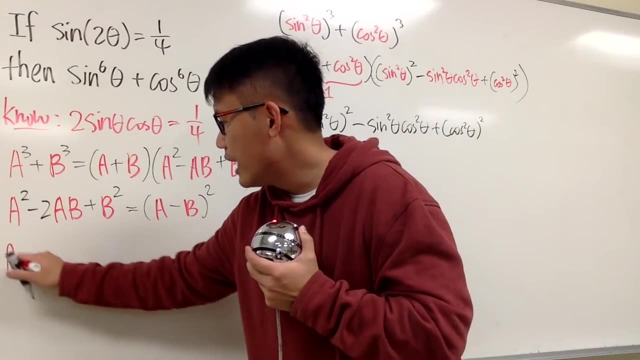 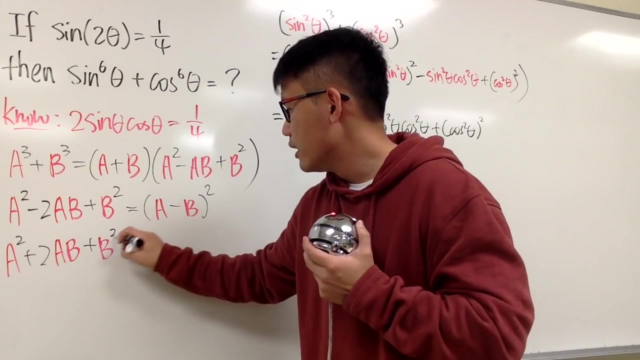 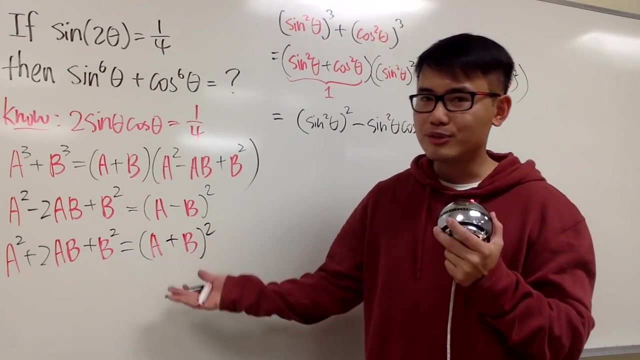 just 1.. So I don't want to look at the subtraction situation. Let's take a look at the addition situation. How's that So similar to this formula? here we know that a squared, if we have plus b squared, this is going to be a plus b, and we square that. This is going to be much. 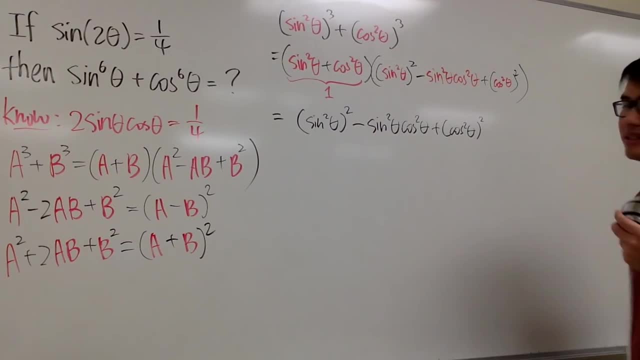 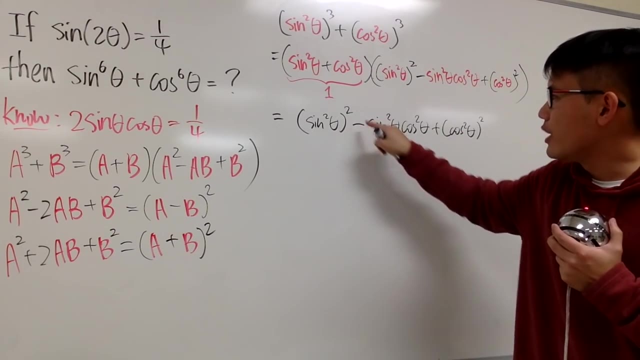 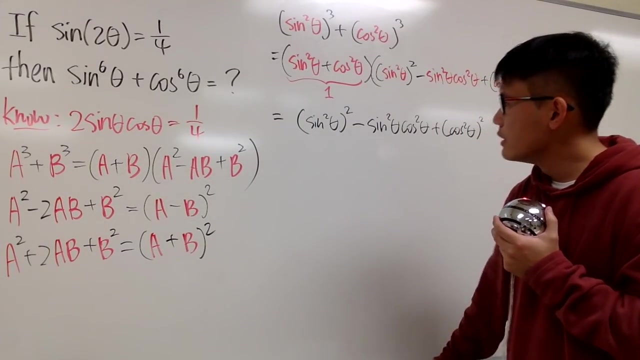 better because, once again, this is my a still. this is my b, still right. So now let's try to make things happen. So far, this is a squared minus a, b plus b squared. okay, And this is what I want to end up with. This is minus 1, right. This is like minus 1 in front, right. 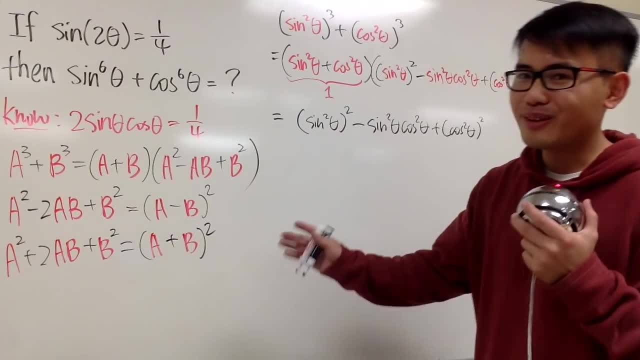 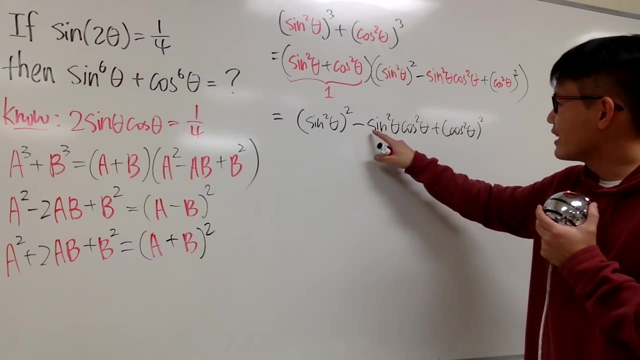 here And I wish to have plus 2, right, That would be so nice if we do have the plus 2.. So how can I make that happen? Well, this is minus 1, right, 1 times sine squared theta. 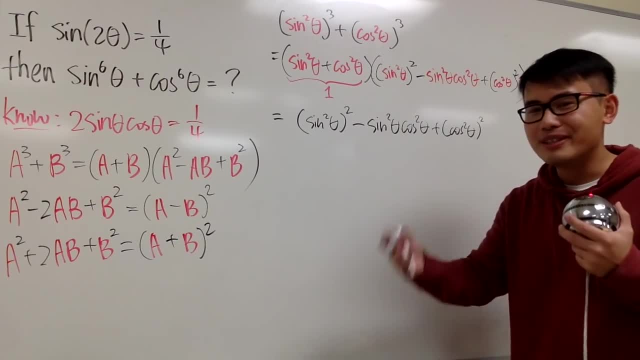 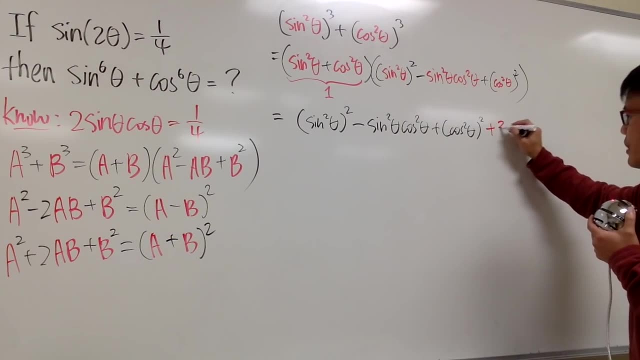 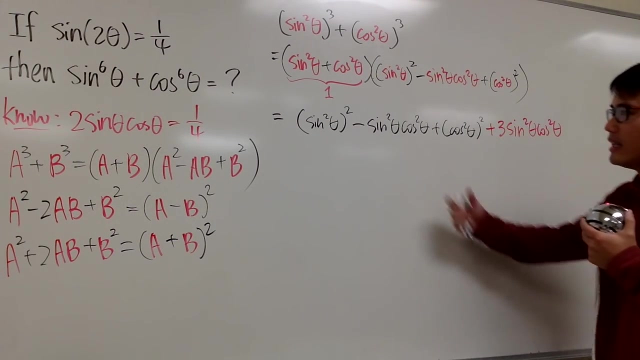 cosine squared theta. Why don't I just add 3? Because negative 1 plus 3 is plus 2.. So look at this term. Let me add 3: sine squared theta, cosine squared theta. If I combine these terms and that term together, I will end up with plus 2: sine squared theta, cosine squared. 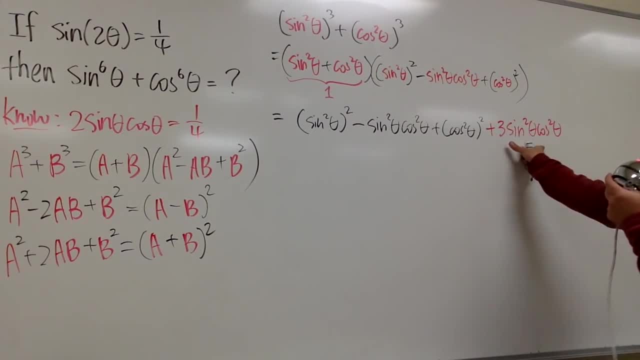 theta right That's so nice. However, I cannot add this to that right. But if I subtract the same thing right away, let me minus 3: sine squared theta, cosine squared theta. If I do that, I can pretend nothing happened, because this and that together is just 0,. 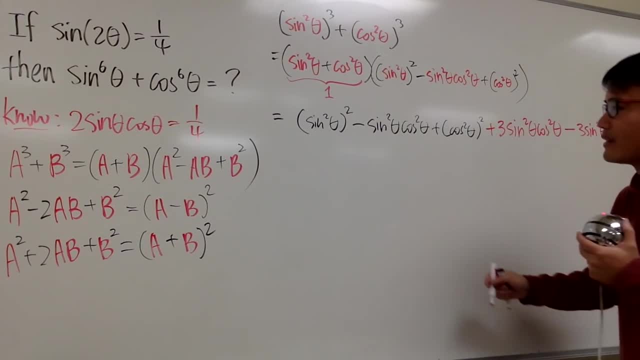 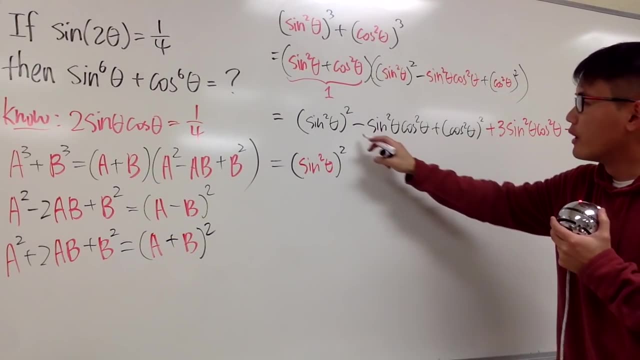 okay, And now let's keep going. Okay, Let's keep working this out. So let me put this down for you guys. now, First term, let me just do it right here: Sine squared theta and I'll square that And for this and that. 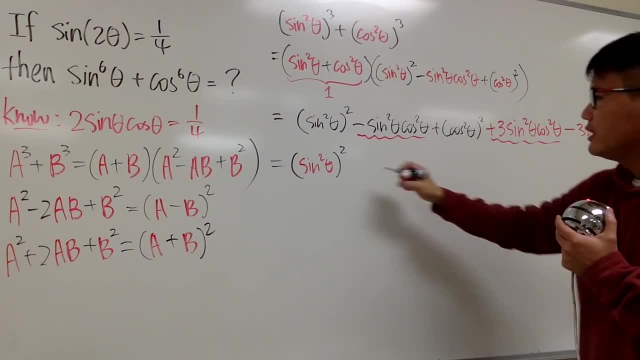 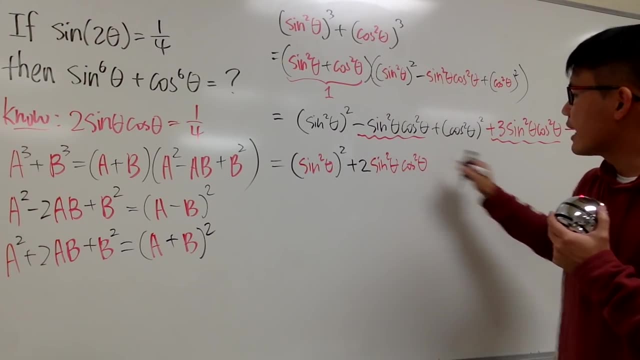 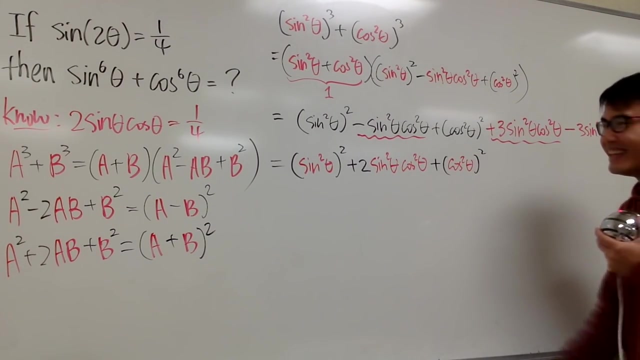 I'm going to combine the terms Negative 1 plus 3 is plus 2.. So I'll put down plus 2.. And then we still have the sine squared theta, cosine squared theta. So nice. And then let me bring down this term: plus, cosine squared theta, and then square. Okay, And now you see. 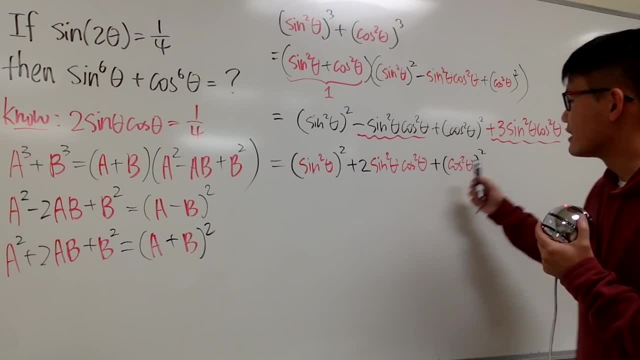 based on this right. Let me fix this right here. We have the a squared plus 2ab plus b squared, which matches 2.4, right, And of course, at the end- don't forget this- right here We still have the. 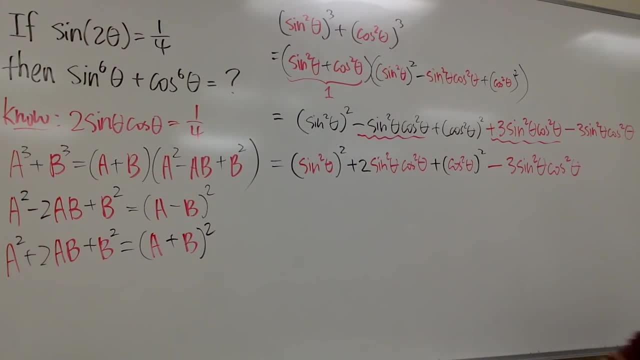 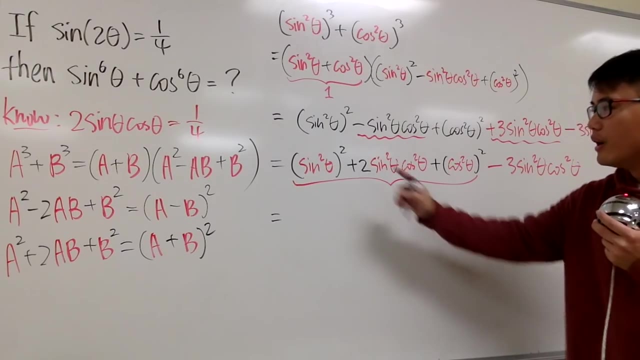 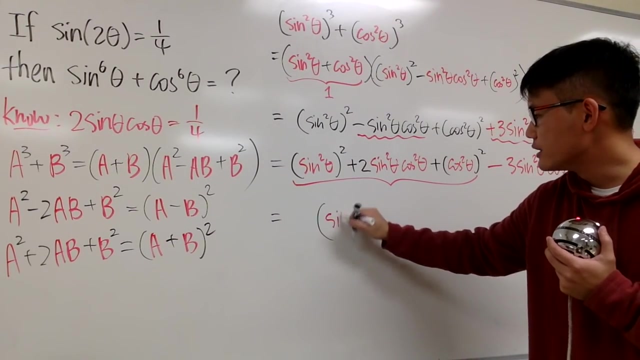 minus 3. sine squared theta, cosine squared theta right here to worry about. Alright, let's see For the first 3 terms right here: a squared plus 2ab plus b squared is exactly a plus b and then squared. So I can write this as a, which is sine squared theta, and. I add it with b, which is cosine squared theta, and add it up to b, which is sine squared theta, plus 2ab plus b squared. So I have this here, And then this is 4 times 2b plus 3b. So right, 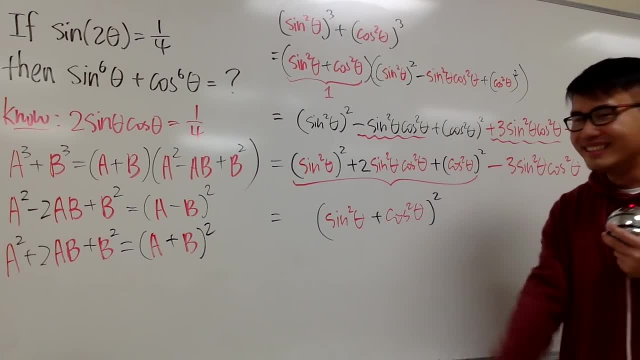 and then I square that. So nice, isn't it? Because once again you end up with 1.. Now, of course, let me write this down again: Minus 3, sine squared theta, times cosine squared theta, All right. 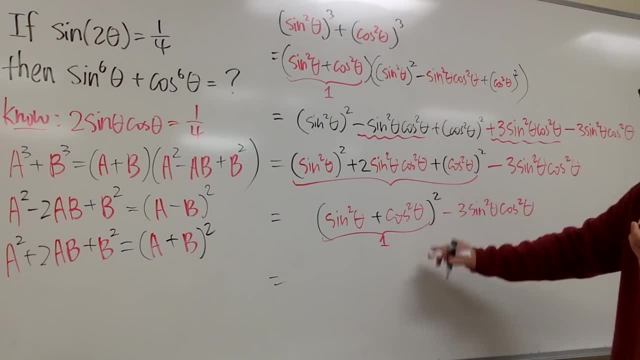 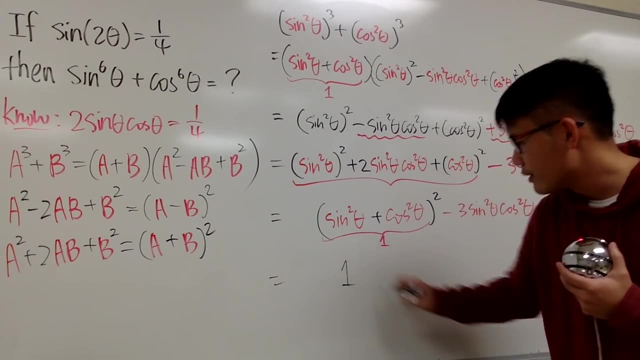 This time, as I said, this is 1.. And when you do 1 squared, you still end up with 1.. But then this is the number 1.. You have to subtract this term right, So we still have to write down the 1, right here. 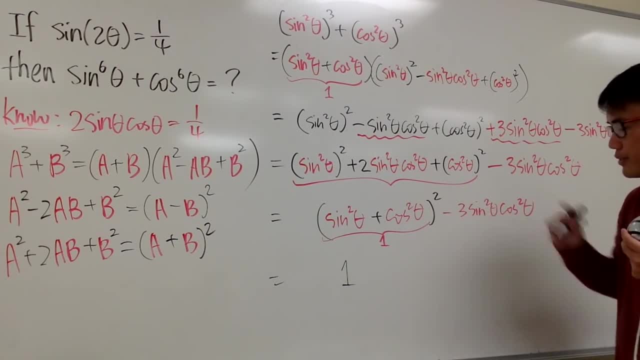 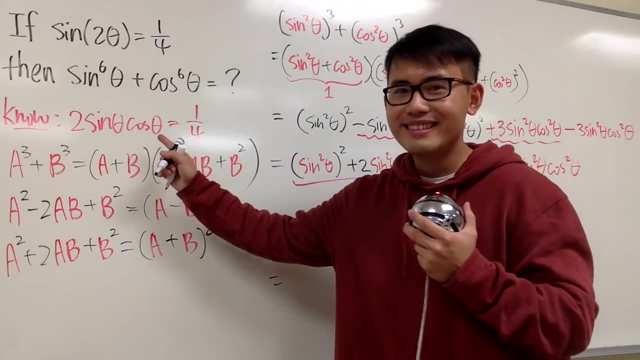 Okay, So this is just 1.. That's good. This is minus 3.. And now we have sine squared theta, cosine squared theta. So let's come back here again. Let's look at this. This is what we know from the original right. 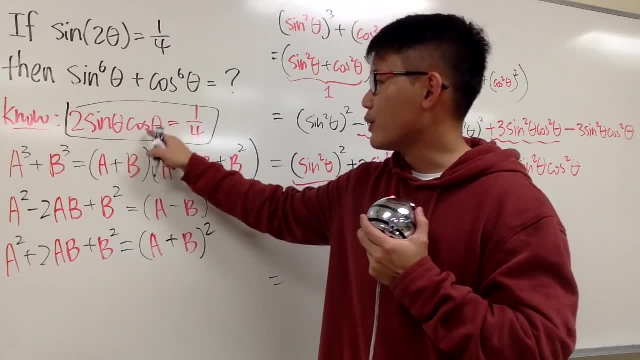 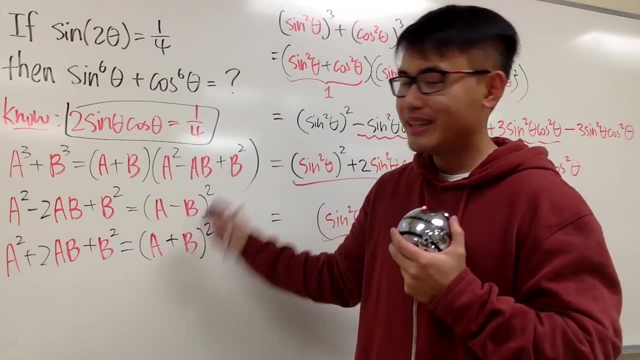 We know 2. sine squared theta, cosine squared theta, is equal to 1 over 4, right? Well, if you look at this and divide both sides by 2, you will get sine squared theta. cosine squared theta is equal to 1 over 8.. 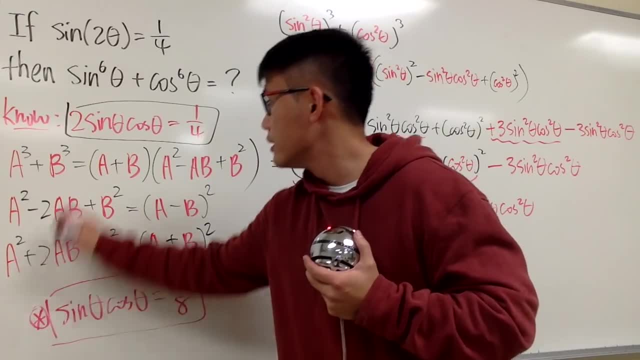 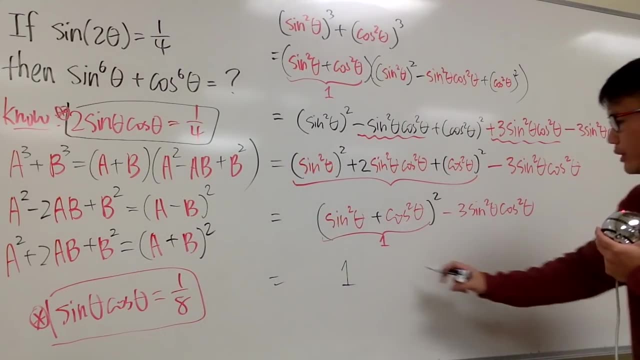 All right, Let me just put this down right here: Divide both sides by 2. And this is what we have right, This and that. Well, let me write this down: Minus 3, sine squared theta, cosine squared theta. 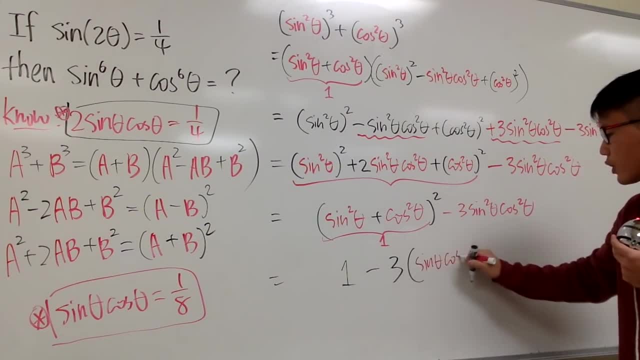 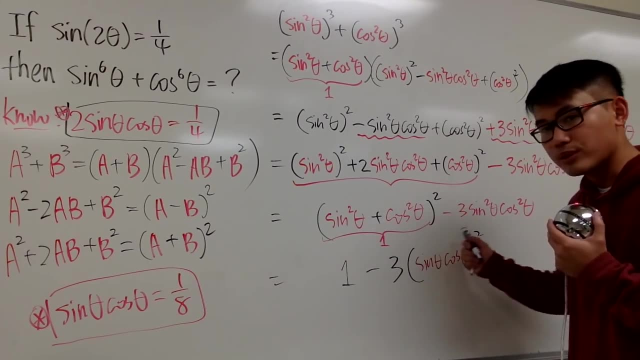 I can write it down as sine theta inside cosine theta, inside of a parenthesis and then square. And the reason I want to do that is I know sine theta times cosine theta. This is just 1 over 8. So we are almost done.